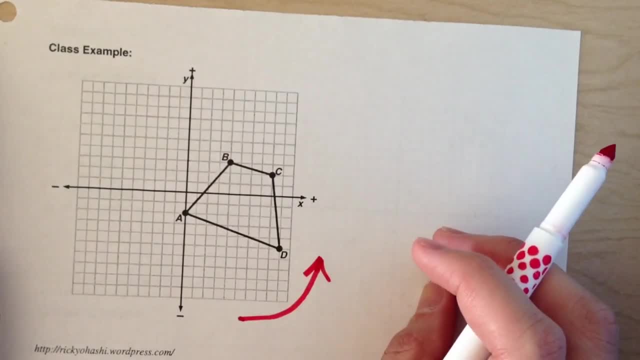 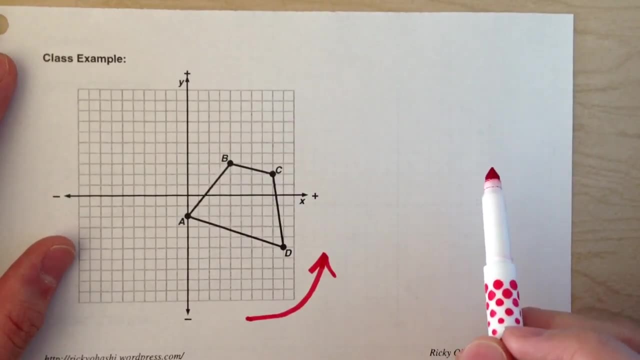 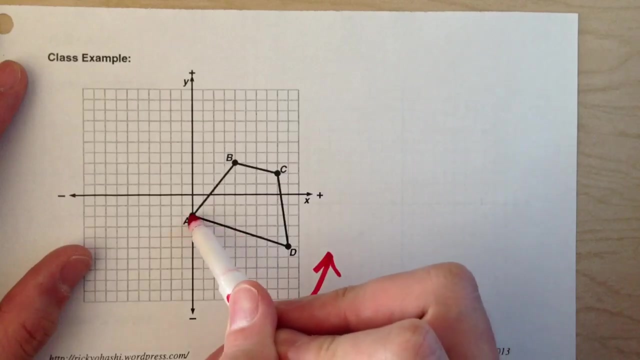 I'm rotating because that's going to come in handy when I'm turning paper all over the place. But one of the first tips you can use is rotating the points on an axis first, For example point A. Rotating this 90 degrees counterclockwise is easy because it's going to end. 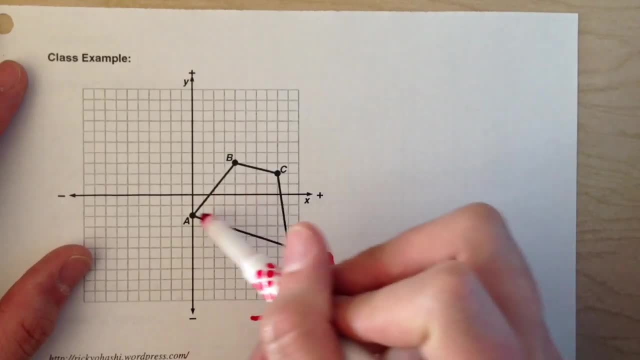 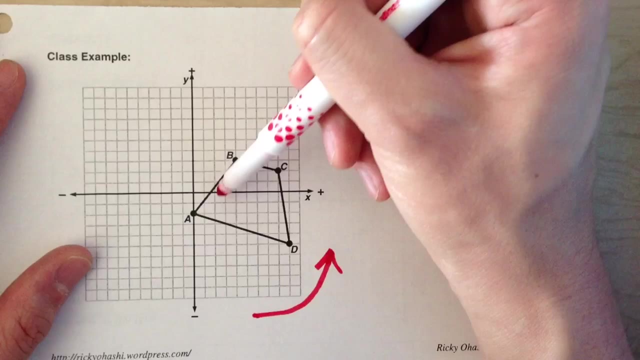 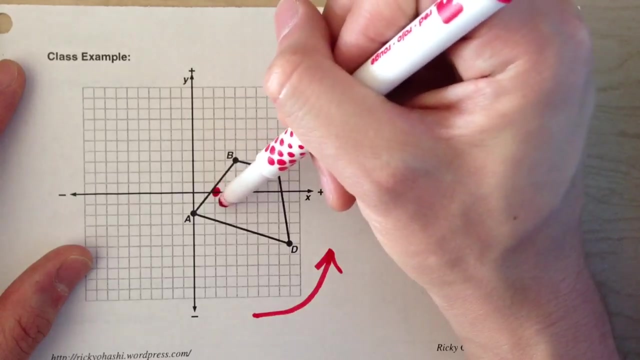 up on the axis next to it. It's just going to rotate onto the next axis, So right now it's two steps away from the origin. When it rotates counterclockwise 90 degrees, it's going to end up two steps away from the origin, while on this axis. Okay. 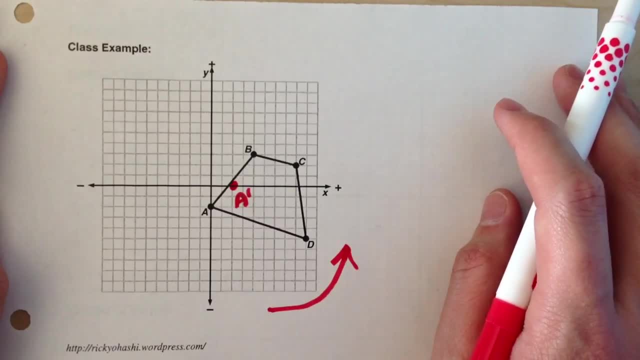 However, the other point is that you can rotate the point 90 degrees counterclockwise. The other points aren't going to be as easy because the other points aren't on any of the axes. So I've got another trick you can use to figure out where those are going to go. 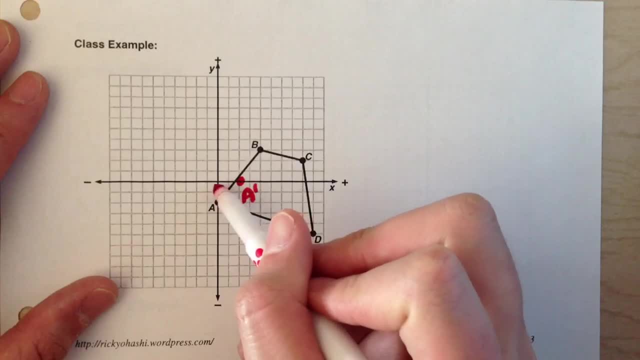 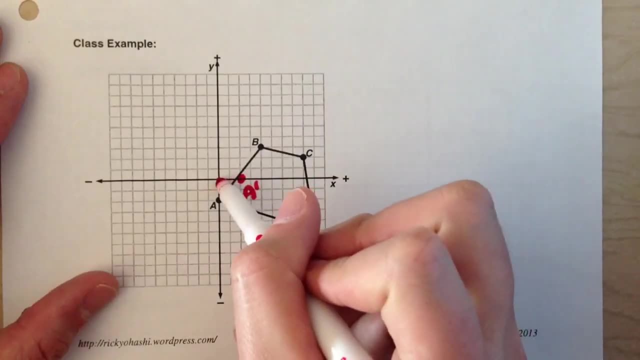 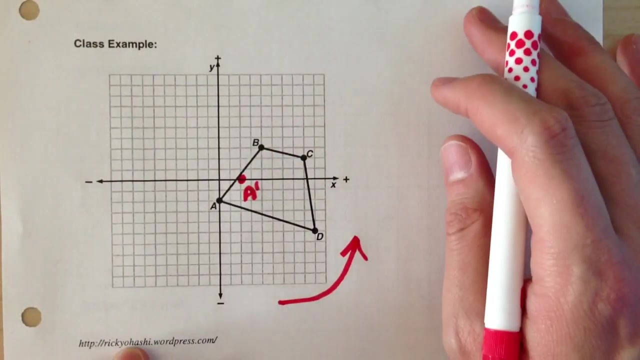 I'll do point B. Notice how point B right now is four steps to the right and three steps up above the origin. So from the origin, four steps right, three steps up, To figure out where B prime is going to go. what I do is I take my coordinate grid and rotate it. 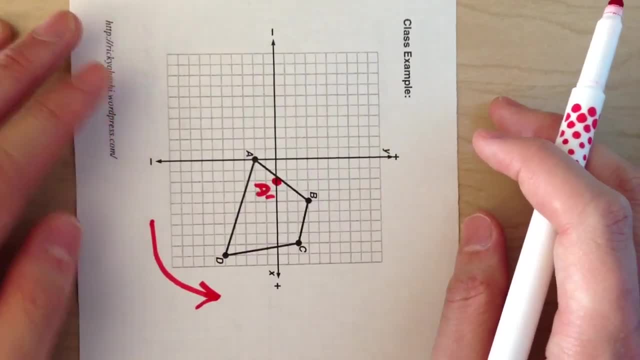 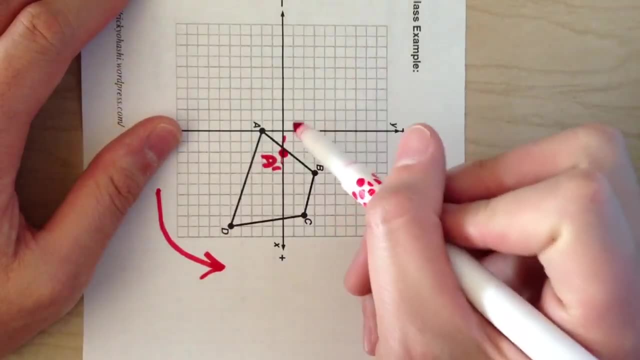 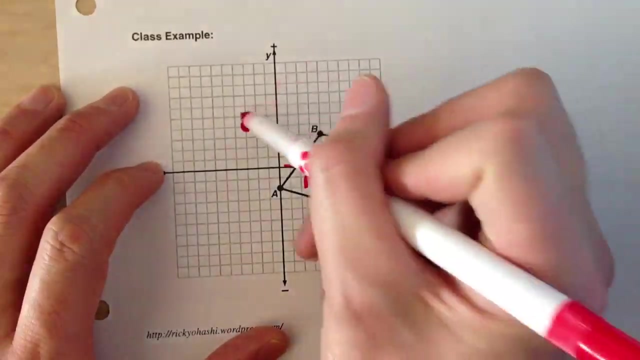 and then follow that exact same pathway that I had before. So remember it was four steps to the right and three steps up. If I rotate my paper from the origin and go four steps right and three steps up, that's where B prime is going to be. 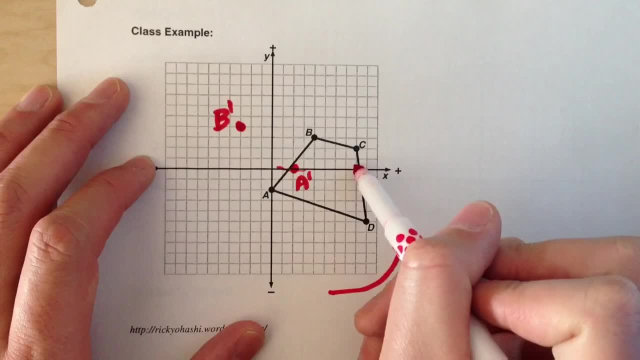 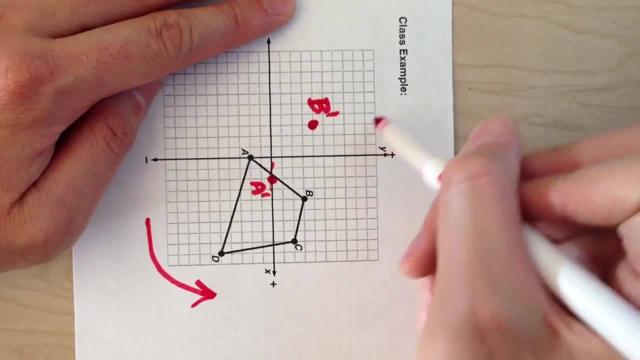 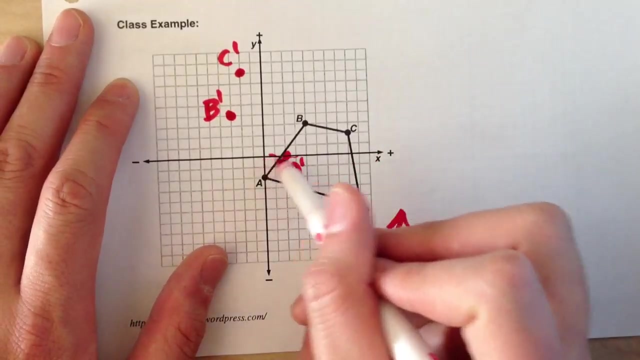 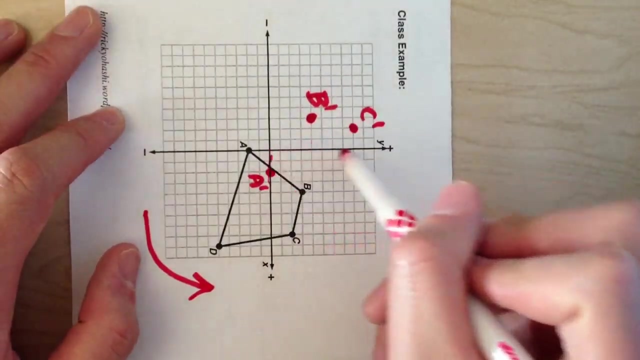 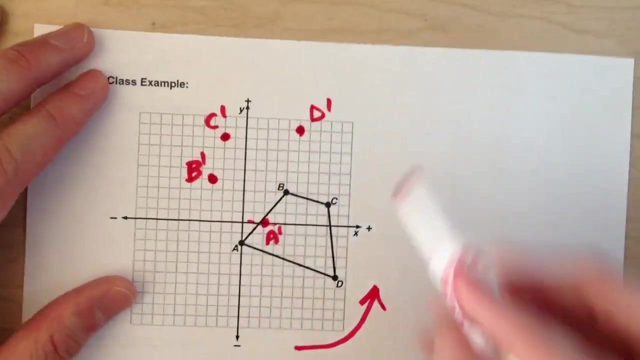 Now let's do C. C is eight steps right and two steps up. Rotate my paper right, 2 steps up. There's C prime. D is going to be 9 steps right, 5 steps down. Rotate my paper 9 steps right, 5 steps down. That's D prime. If I connect my dots, that gives 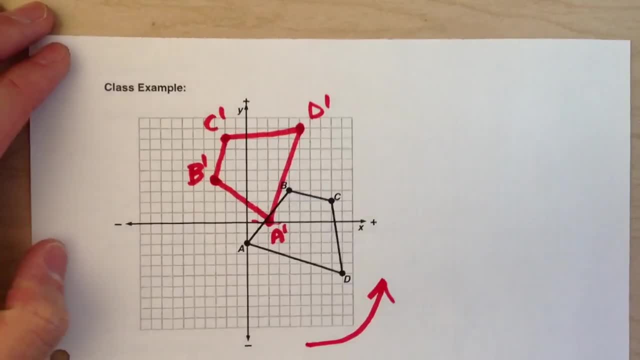 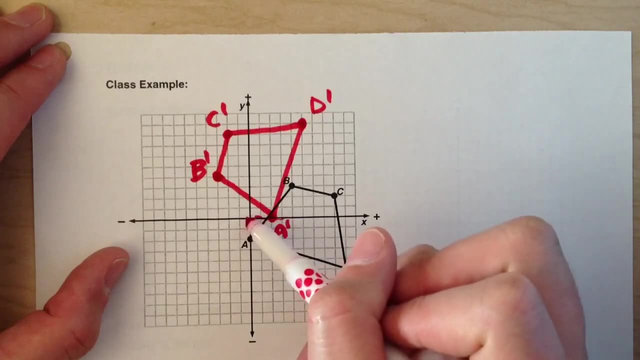 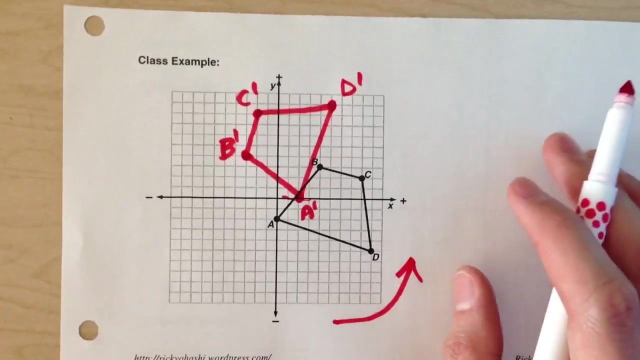 me my rotated trapezoid. So the key to doing this is basing on the origin. find a path that goes from the origin to your point and then rotate your paper and repeat that path. Alright, good luck.